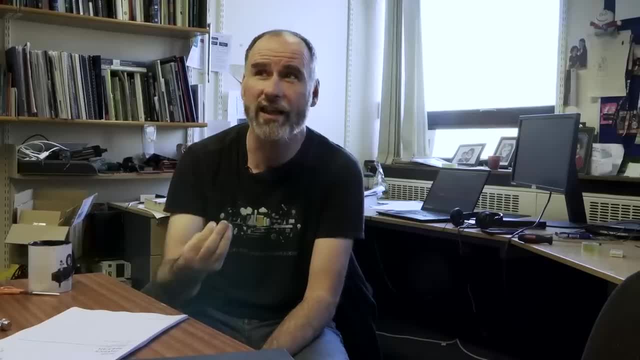 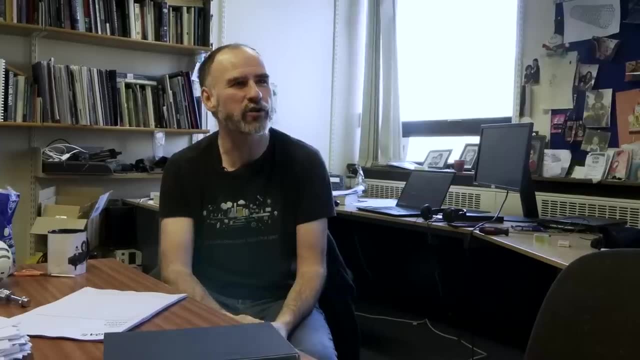 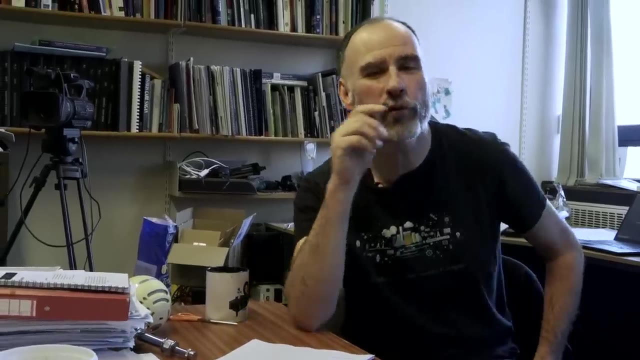 What I want to do is see to what extent it has any intuition or anything that we expect of our students in terms of: does this answer make sense And does the reasoning here make sense? We'll look at the most basic question first, but before we do that, can we do something that's fun? Let's get. 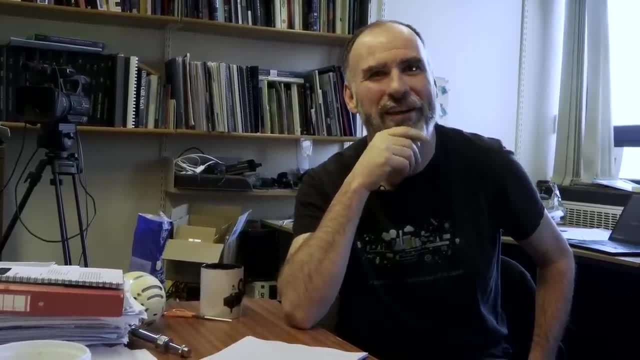 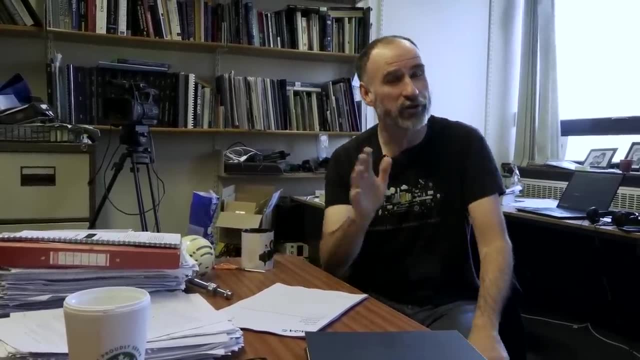 it to generate a mission statement for the University of Nottingham, Just to show you we're going to be talking about maths and we're going to be talking about physics concepts. but let's just see how it does. Let's see how it does on the stuff that it's really, really good at. 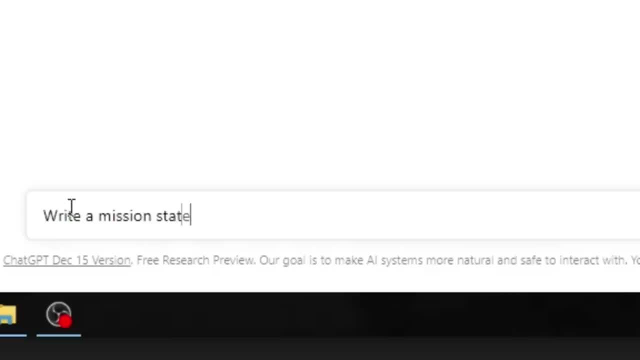 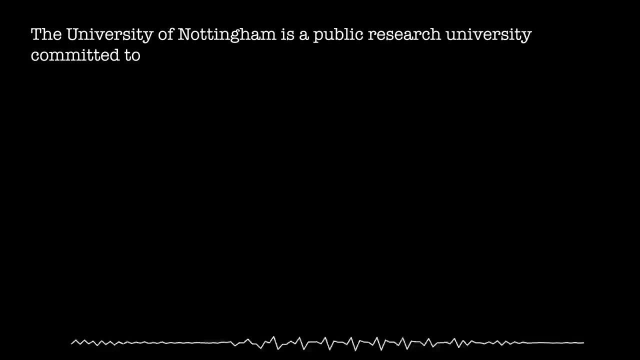 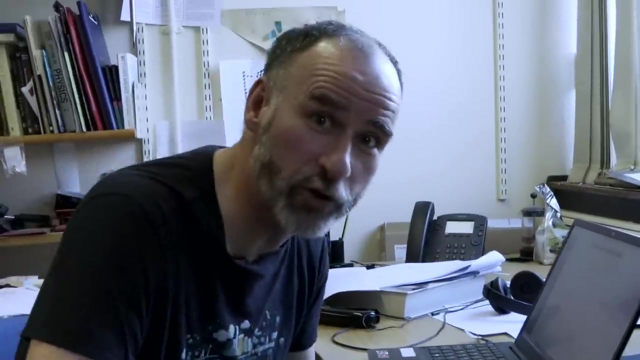 Write a mission statement for the University of Nottingham. The University of Nottingham is a public research university committed to excellence in teaching and research Committed to excellence. Is there any word more nebulous than excellence? What else are we going to do? Strive for mediocrity? 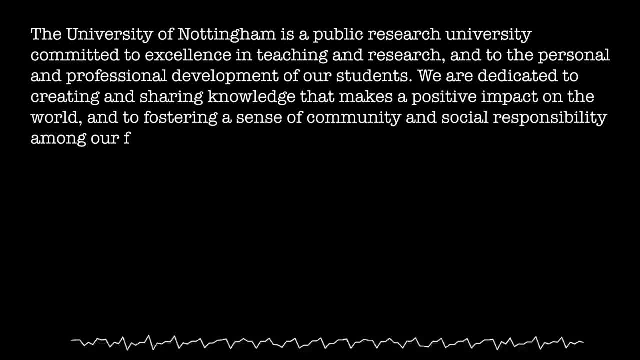 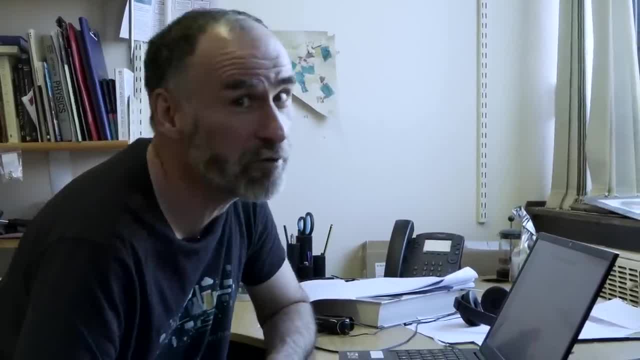 And to fostering a sense of community and social responsibility among our faculty staff and students. But this is the mission statement. This is exactly the type of blurb you get from every university, not just in the UK. These things are interchangeable. You can take the University of Nottingham off there and just replace it with 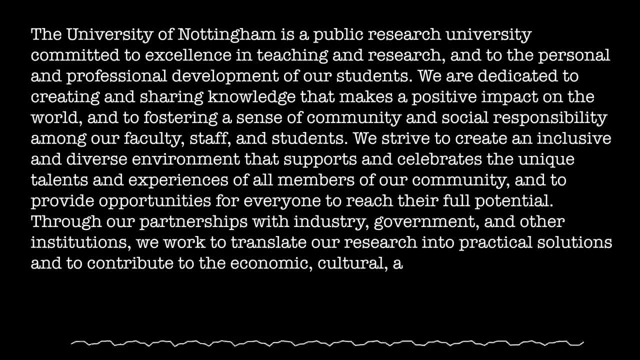 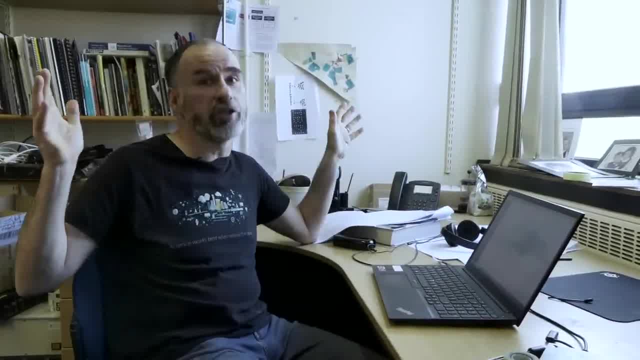 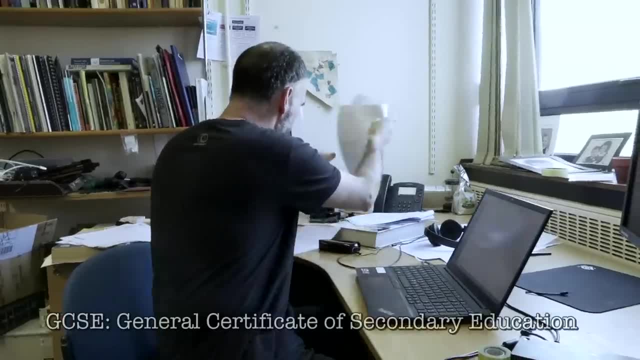 anything else, We work to translate our research into practical solutions and to contribute to the economic, cultural and social well-being of our region and beyond. So let's start with a GCSE question. So this is middle school, relatively low level. Let's see how well it does if I can find my GCSE papers somewhere. 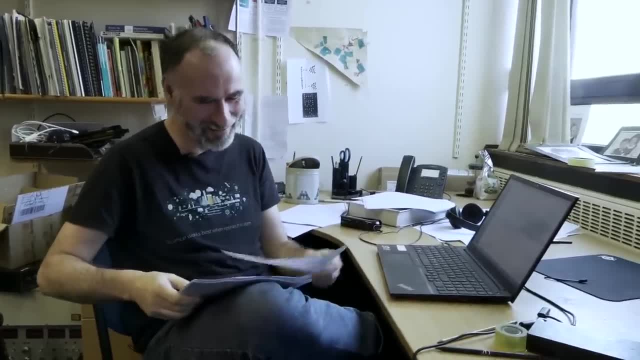 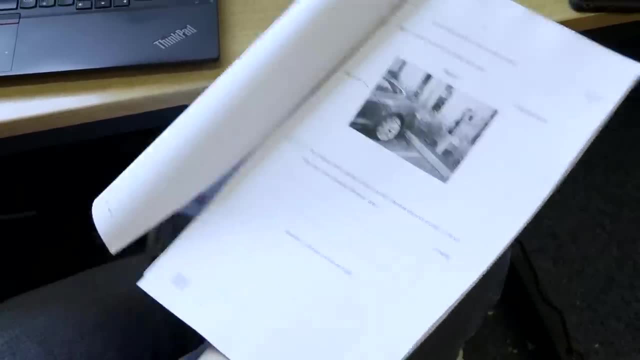 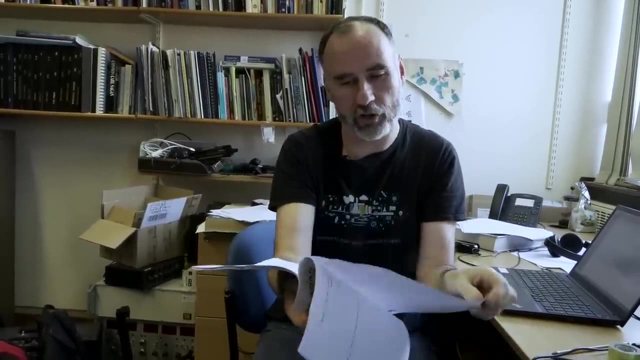 Thank you, Sean. As if by magic. So this is paper one, So it's an electric car being recharged. So now an interesting thing: Lots and lots of diagrams, Lots and lots of diagrams, Another diagram, And it's all about interpretation of those diagrams, And this is not just for 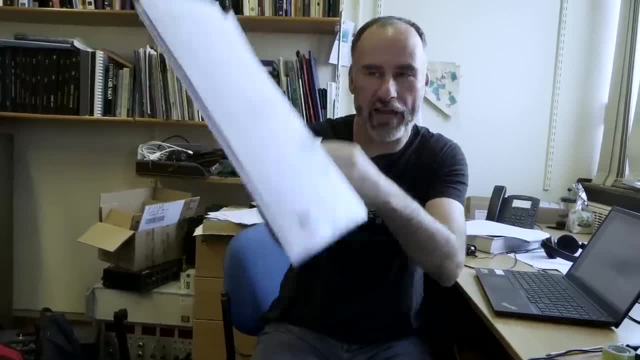 middle school or GCSE physics. This is across the board: Diagrams, Diagrams. So, with chat, GPT being text at the moment, it doesn't have the facility to do that. It doesn't have the facility to do that. It doesn't have the 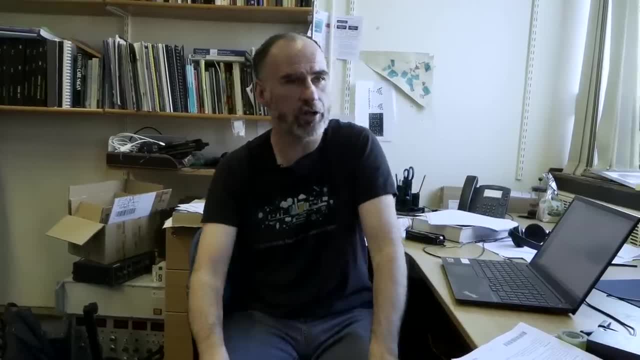 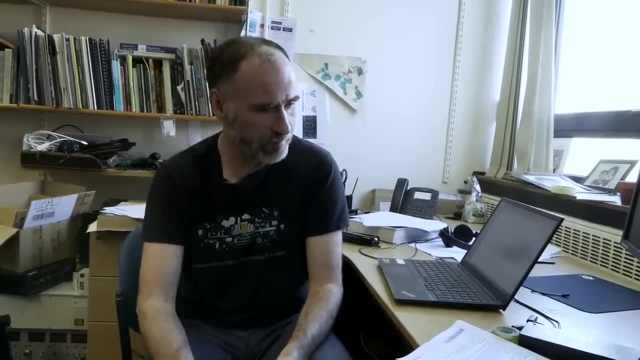 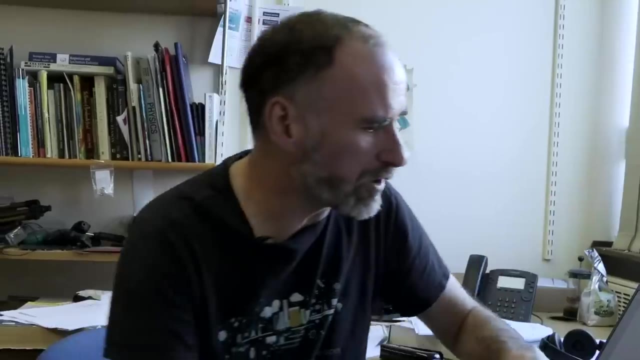 facility to really parse those and extract the information. When it does have that facility- and that would be a remarkably powerful facility- it will be extremely impressive, So assuming it does the interpretation correctly. So let's choose one. So that means we're sort of limited in our options, But let's choose one. Question one actually in this paper. The battery in an electric car can store 162 million joules of energy. The charging station has a power output of 7,200 watts. Calculate the time taken to fully recharge the battery from zero. So I'm going to type that in. 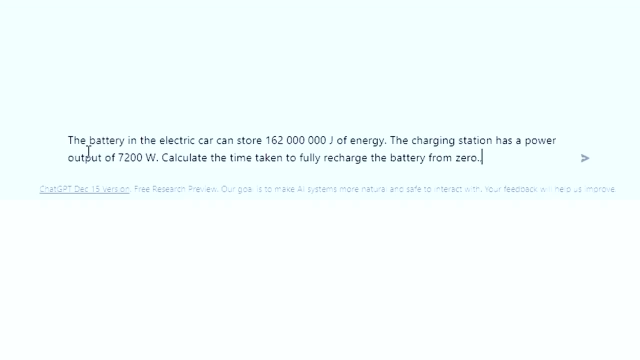 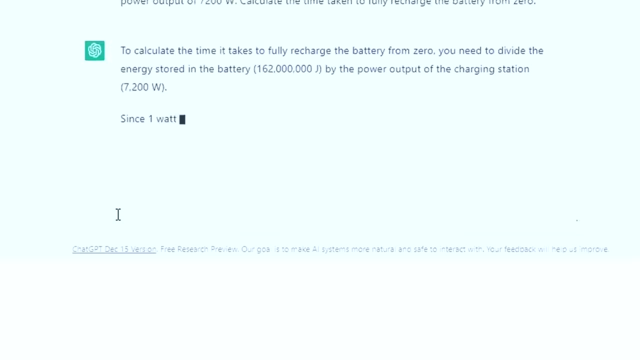 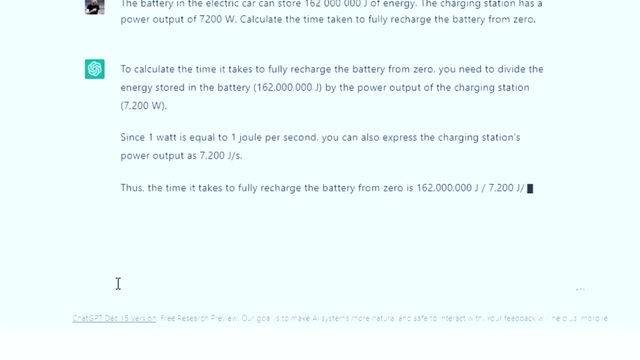 Let's grade them as well. So this one's worth three marks. Go for a chat. GPT, Thinking, Thinking. Good start. To calculate the time it takes to fully recharge the battery from zero, you need to divide the energy stored in the battery by the power output of the charging station, Since one watt is equal to one joule per second. 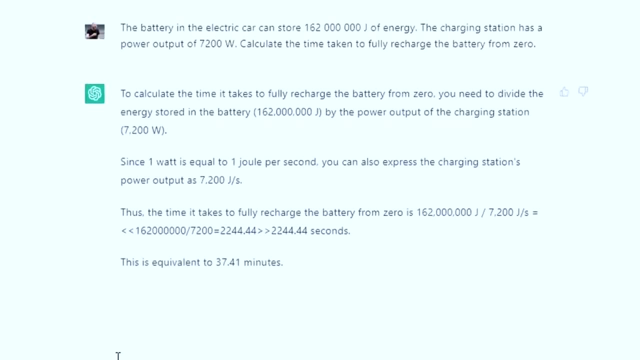 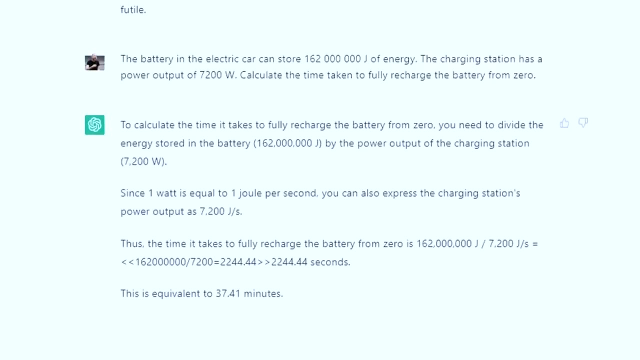 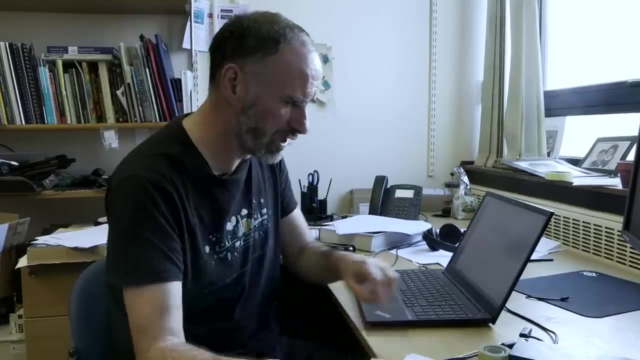 you can also express the charging station's power output as 7,200 joules per second. Thus, the time it takes to fully recharge the battery from zero is Which it says is. What's interesting here is that the reasoning is correct, but I'm not certain that number is correct. 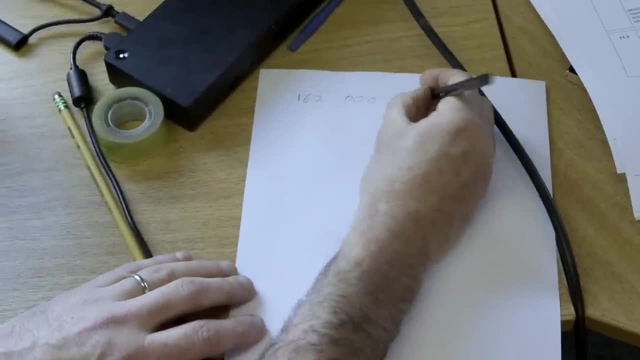 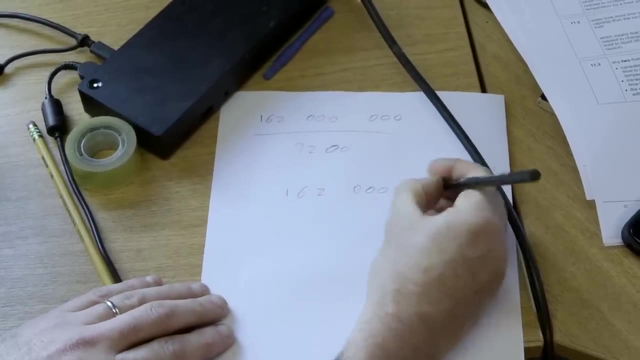 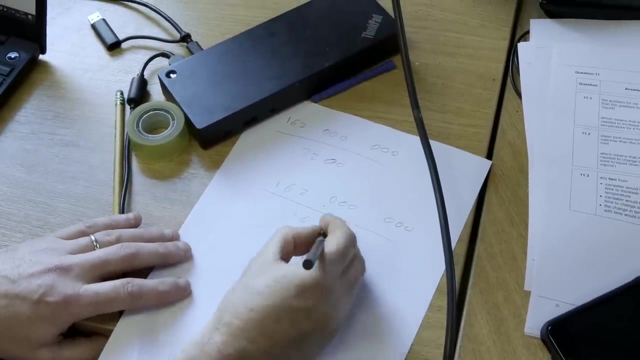 We do what all good physicists do: You always look at that answer and make sure that that answer makes So มา цию. we'll round it up just to get a ballpark figure, It should be greater than 16,200.. 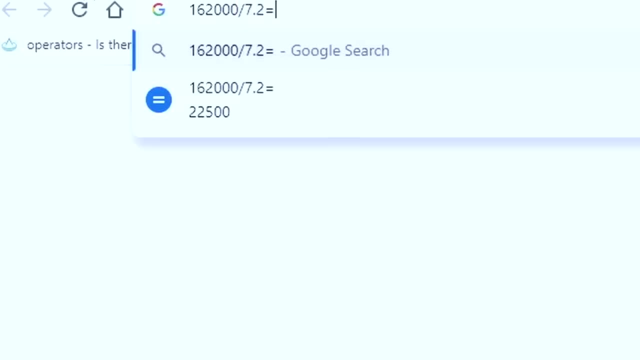 It looks like it's lost a factor of 10.. Yeah, it's out by a factor of 10.. Now that's intriguing, isn't it? It gets the reasoning correct. I guess it's language. it's a language model. 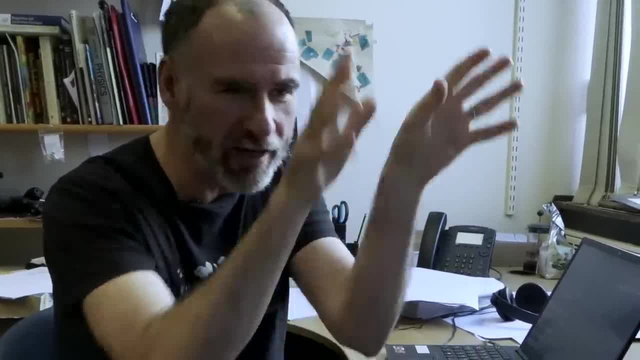 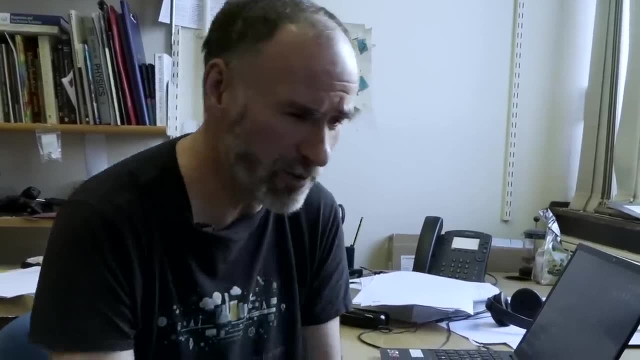 It's making predictions based on the correlations between words and a sentence. I'm not entirely certain, I've got to admit, how it handles maths. Maybe we can come back and have a whole video about that, Sean, But that is intriguing that it gets the reasoning correct. 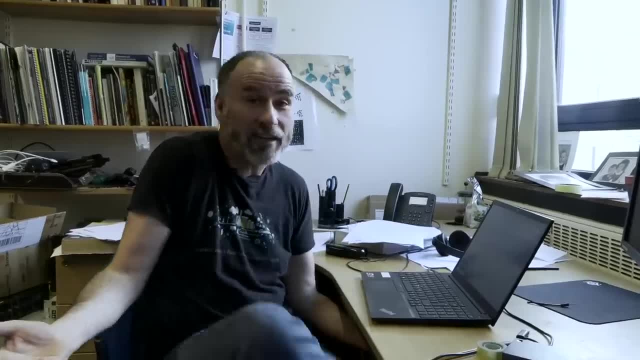 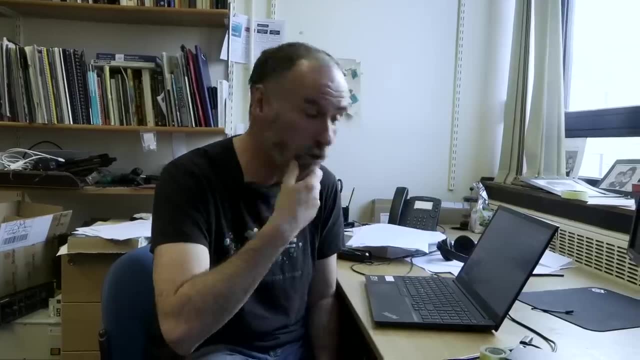 and drops a factor of 10, like all of us do. That's exactly the type of mistake I would make. I spent my life correcting for factors of two and factors of square root two, So that's intriguing. So, given that there's three marks for this, 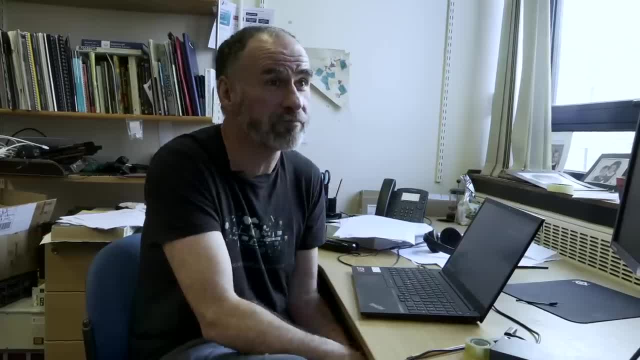 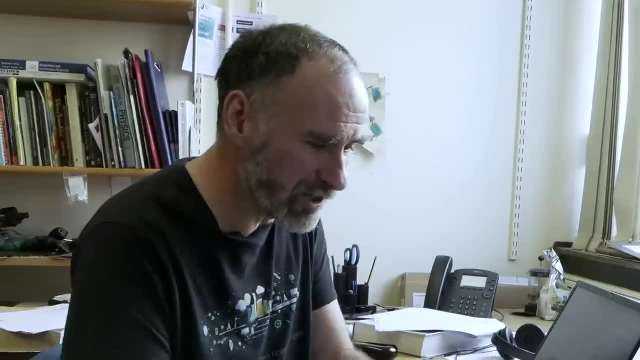 it's got the reasoning correctly. It feels almost unkind to not give it the three marks, but it didn't get the correct answer, So let's say two marks out of three. Okay, let's give it a textual question again from this GCSE sort of middle school. 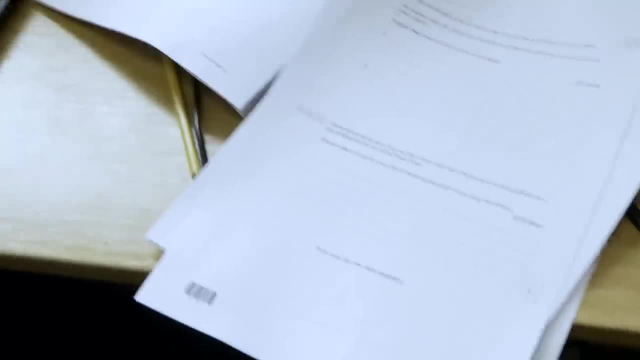 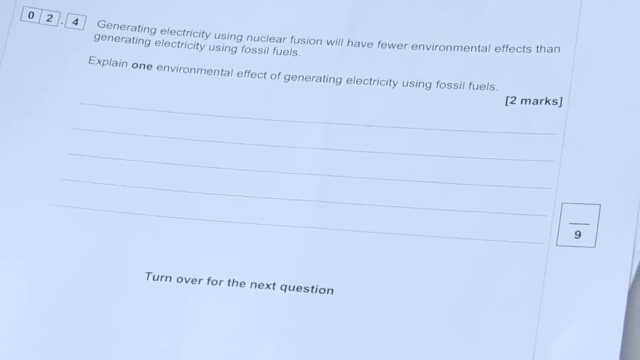 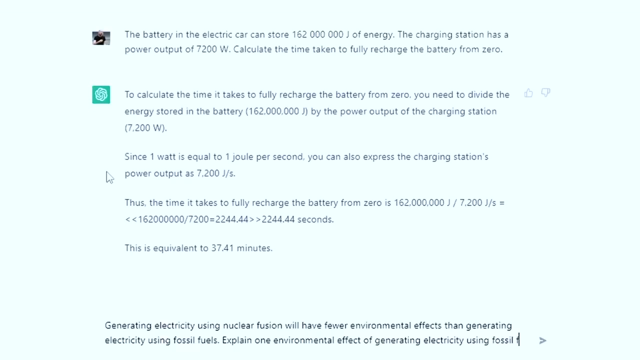 type paper. Generating electricity using nuclear fusion will have fewer environmental effects than generating electricity using fossil fuels. Explain one environmental effect of generating electricity using fossil fuels. Let's see how ChatGPT does on this. Okay, so we can't put the bold in. 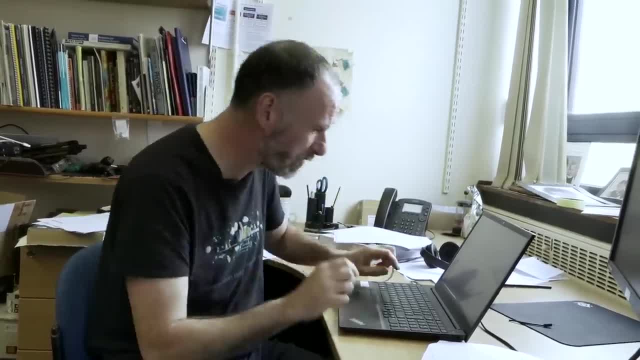 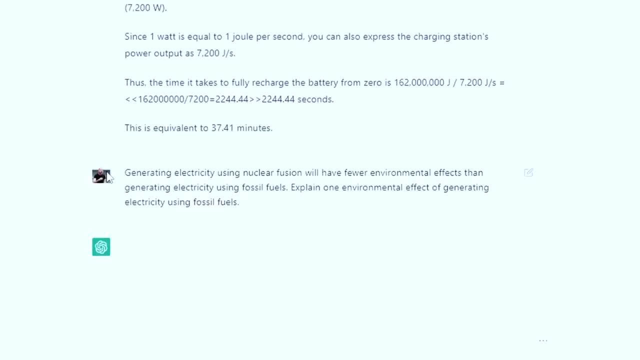 Well, I don't know, maybe we can use HTML and we can put a little B in braces before and afterwards and slash B afterwards, but let's just go with this Thinking. so apparently it's been trained in terms of the ethical considerations. 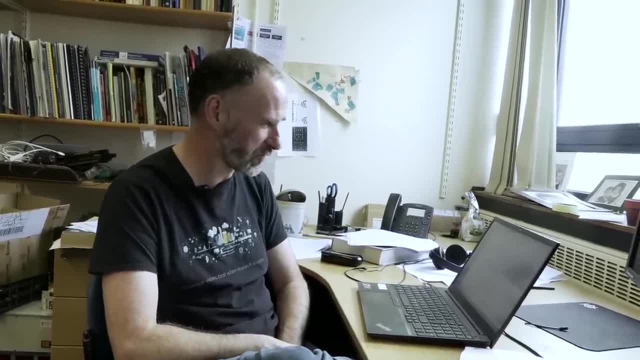 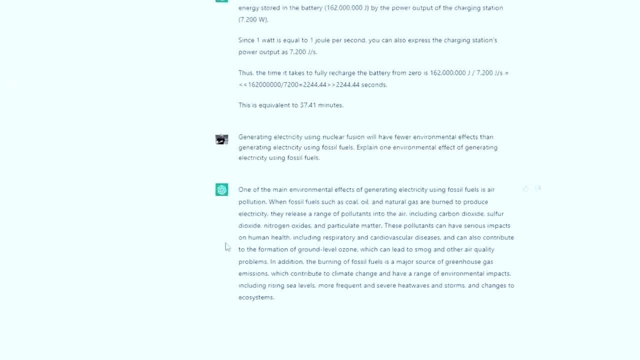 and in terms of misinformation, they have severely restricted it. apparently There are ways around that. however, I guess in terms of you know, you could put it in the context of a novel or something or a fictional scenario. One of the main environmental effects: 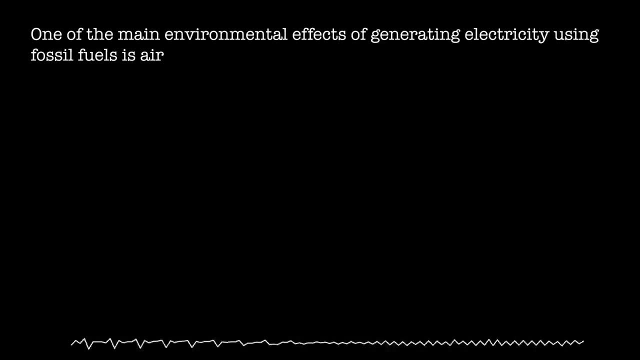 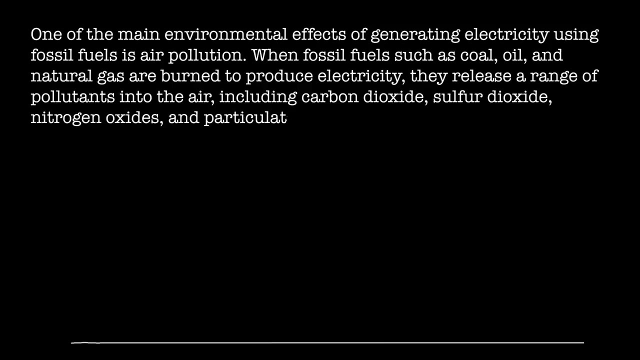 of generating electricity using fossil fuels is air pollution. When fossil fuels such as coal, oil and natural gas are burned to produce electricity, they release a range of pollutants into the air, including carbon dioxide, sulfur dioxide, nitrogen oxides and particulate matter. 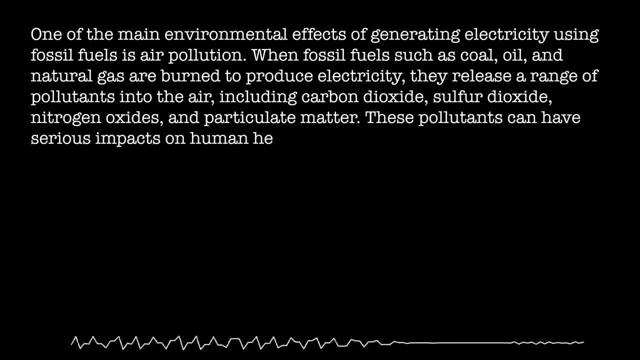 These pollutants can have serious impacts on human health, including respiratory and cardiovascular diseases, and can also contribute to the formation of ground level ozone, which can lead to smog and other air quality problems. Two marks, I think it's fair to say, on that. 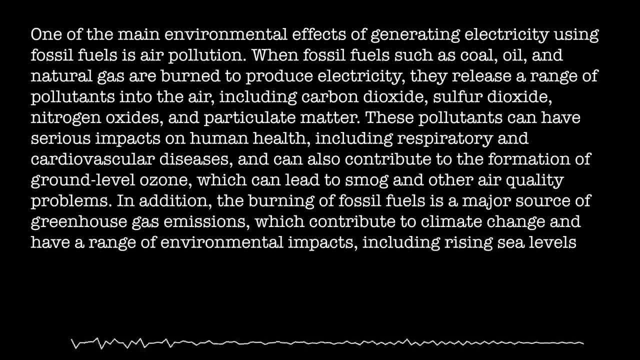 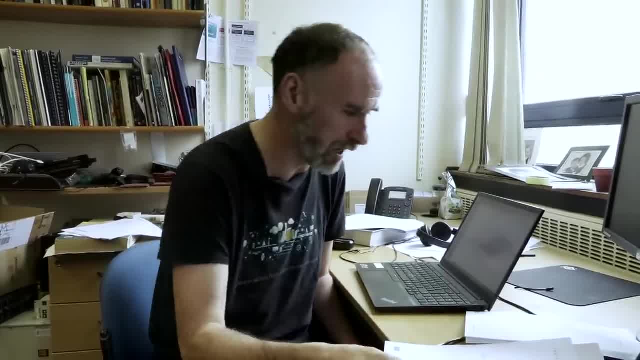 Two out of two for that question. Now we could spend a lot of time on the GCSE questions just going through individual ones. It gets a bit boring. Let's up the level. We're gonna go to A level now, So AP level, so high school level. 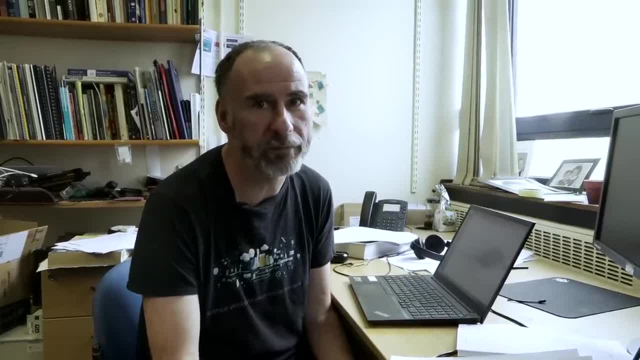 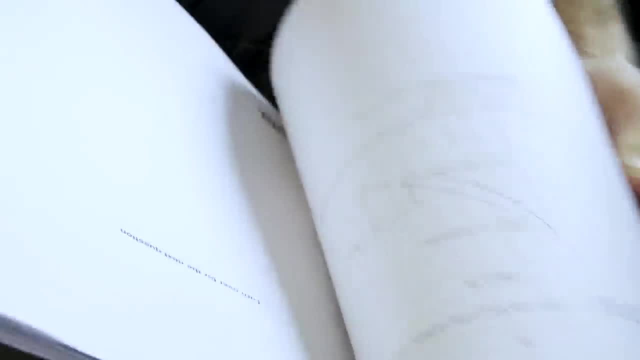 The type of questions that form the basis of exams for entry to university. I think you all know what A levels are. Notice, if I just flick through this, how often we're getting figures. So for all those academics out there, including myself, 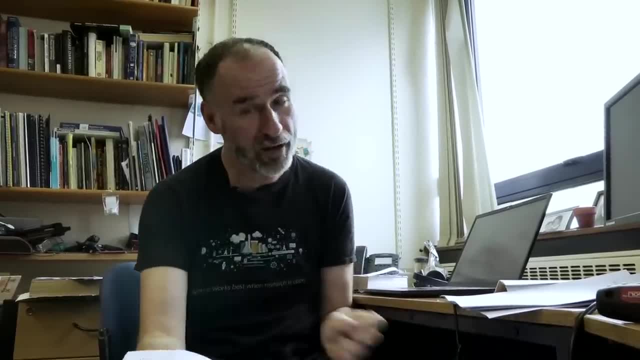 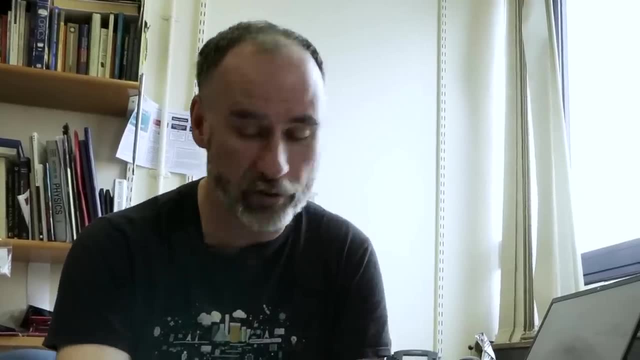 we're going. oh, this is the end of assessment. At the moment, best thing to do is just make sure that it's all about data interpretation. It should be about critical thinking, data interpretation And I think at the moment, if we want to bypass JADCBT, 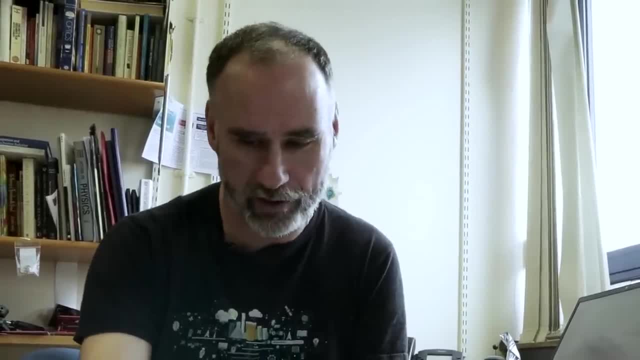 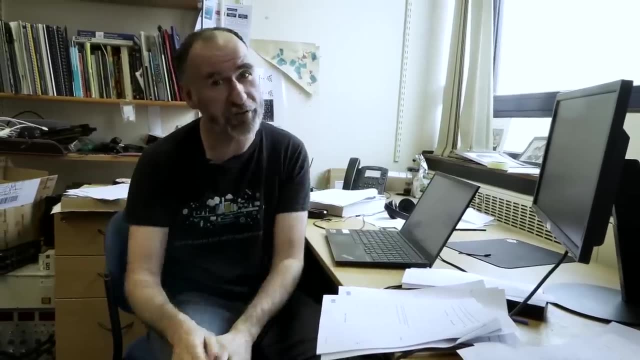 then make sure we put lots of figures in there, make sure it's all about data interpretation. Particle of mass M is oscillating with simple harmonic motion. Simple harmonic motion, the bane of so many students' lives, but it's a very beautiful thing. 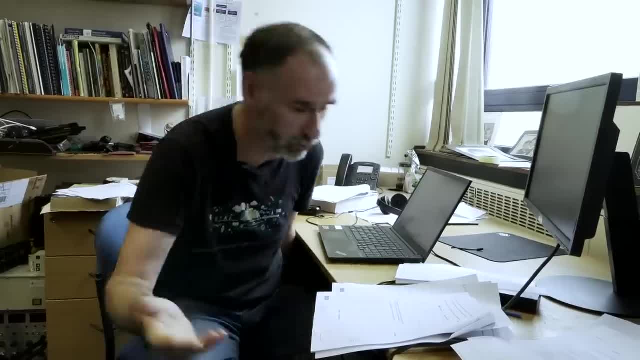 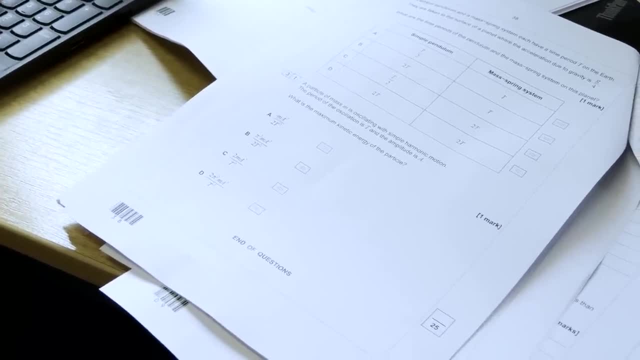 and it underpins so much of physics, including fast sway. It's a quantum field theory for one and quantum mechanics, So this is a very traditional question. as you can see, it's one mark. Let's see how it goes. 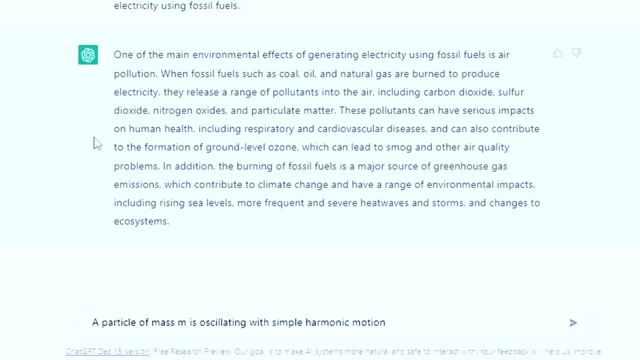 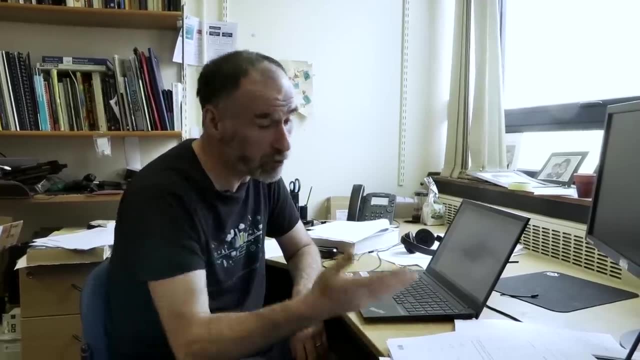 We're not going to give it the multiple choice Motion period- One mark- so it should be able to do this pretty quickly. And actually, for those of you who are physicists- you're doing A-level- you should be able to do that. 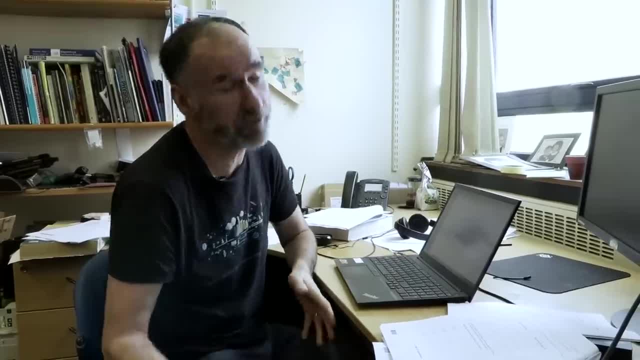 fairly quickly. You don't have to think about causes, you don't have to think about signs: You can think about causes. you can think about signs. you can think about derivatives. you can think about all of that, but all you need is conservation of energy. 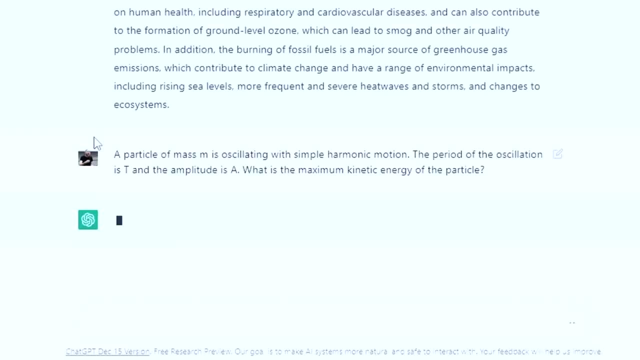 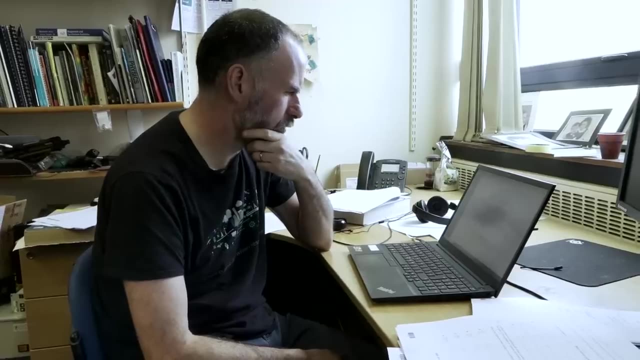 You know this. All you need is conservation of energy to do this. So thinking: Ooh, no, it doesn't, Oh, that's bad At the maximum. no, no, no, no, oh, oh, that's really bad. 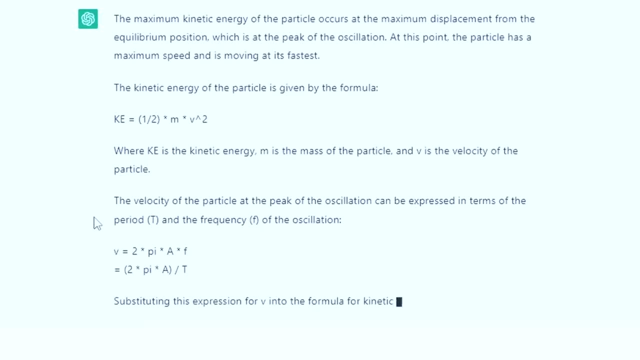 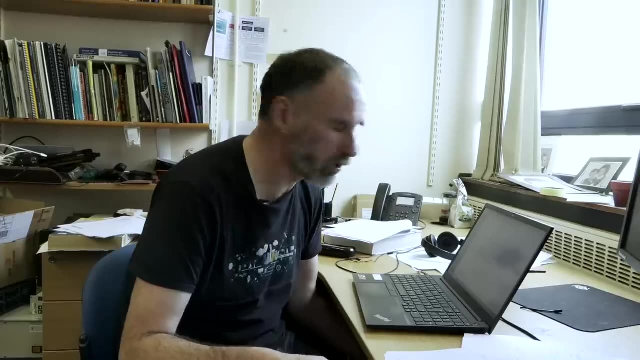 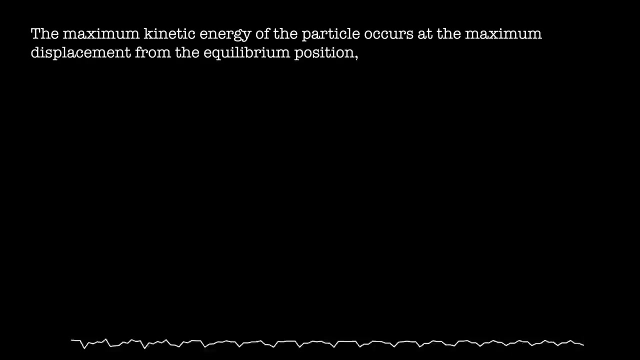 The very first line is nonsense. Yeah, it's interesting, it gets the right answer, but for the wrong reasons. The maximum kinetic energy of the particle occurs at the maximum displacement from the equilibrium. Absolutely not so. that's wrong And regardless of it getting the right answer, 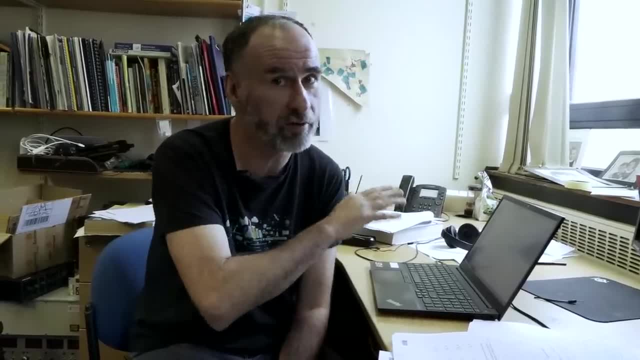 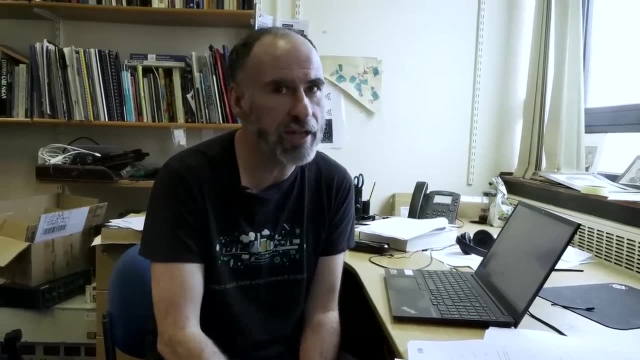 if it were me that were marking this and the students put that down and hasn't crossed it out, I'd be very, very unwilling to give a mark in that sense, because that's a complete misunderstanding of the dynamics of simple, harmonic motion. 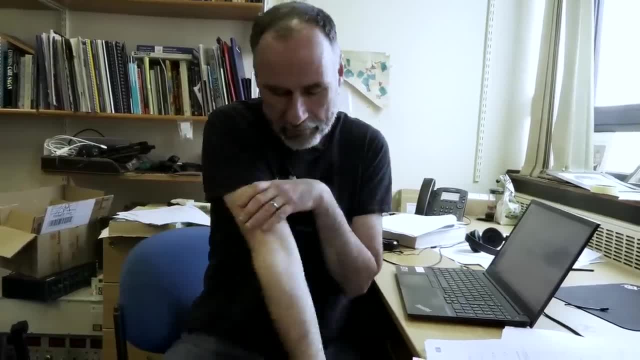 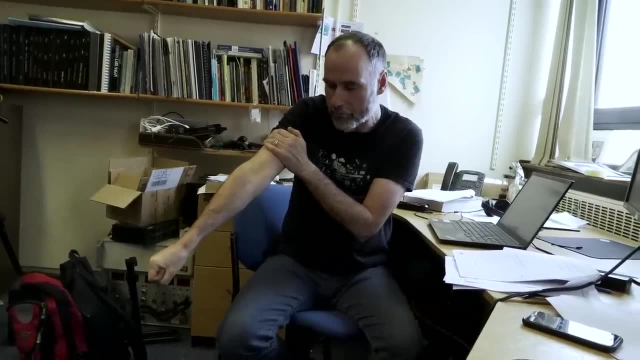 So maximum kinetic energy of the particle doesn't. So basically imagine a pendulum going back and forth. We started off from a fixed position, so it's not moving. So it's got maximum. let me stand up. It's got maximum potential energy here. 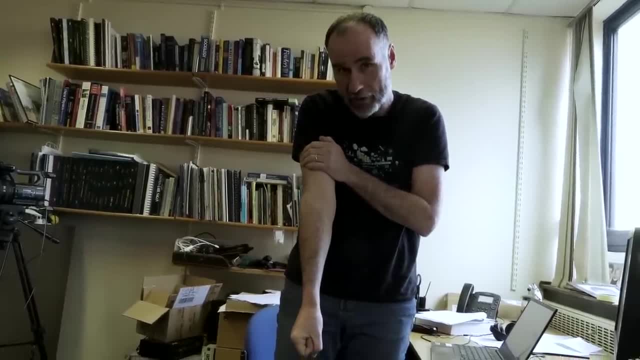 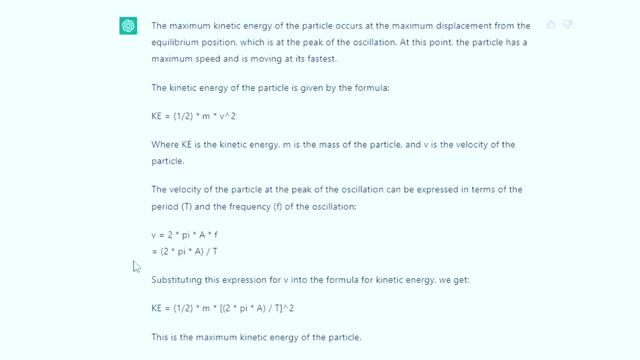 zero kinetic energy, Then it's gonna have zero potential energy here, maximum kinetic energy. This gets it completely wrong. And what's interesting is that that first line is in the context of other stuff which seems broadly correct. It's put the maths down relatively correctly. 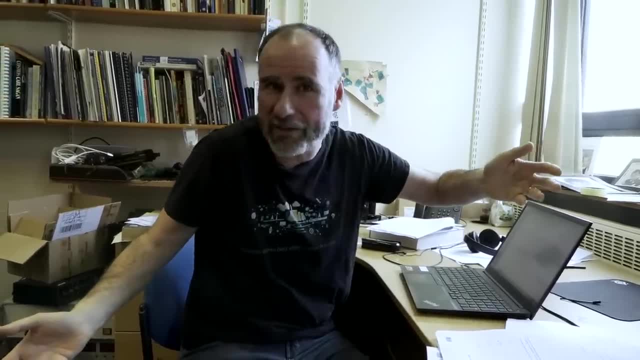 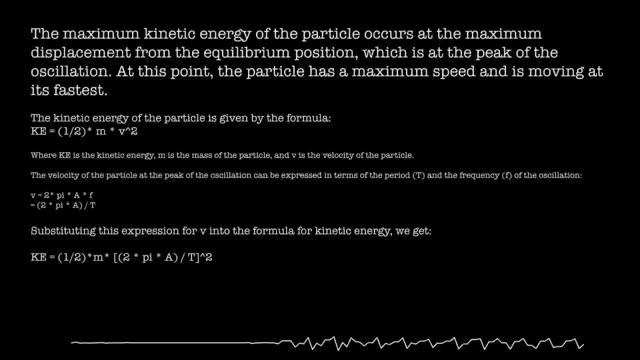 but it doesn't get the physics concept which you wouldn't expect it to. but that's worrying. So for those of you thinking about using chat GPT to do your homework, think carefully. This is the maximum kinetic energy of the particle. 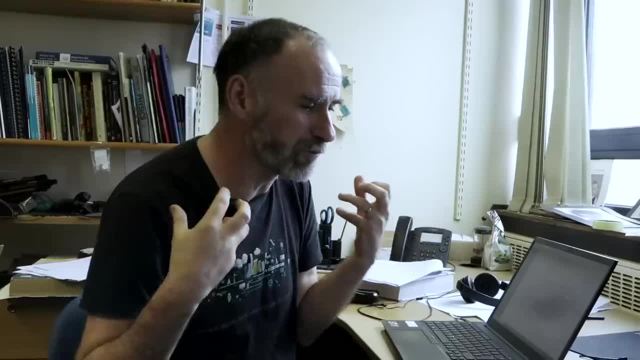 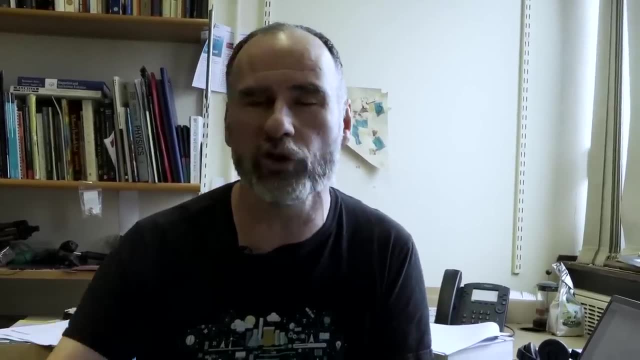 Interestingly, it got the right answer, but for the wrong reason And for us. so in this case I would be less willing to give the mark, And I think a lot of physics teachers would be less willing to give the mark than in the first case, where it got the reasoning correct. 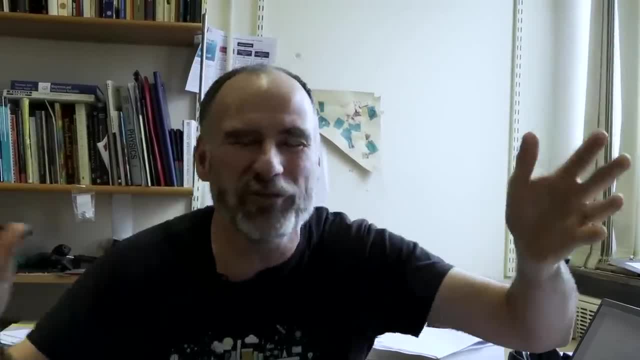 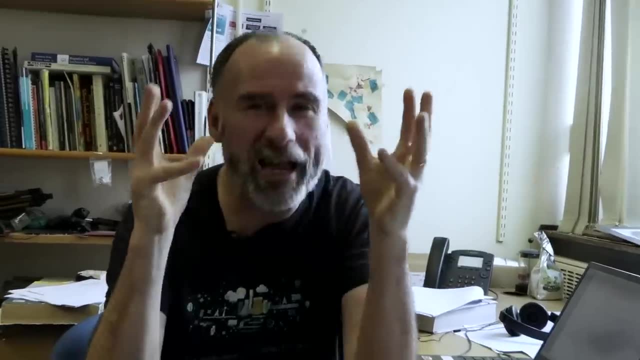 and then it just screwed up. in terms of dividing, That doesn't really matter. Well, it doesn't matter if you're sending probes to Mars or whatever. you don't wanna be out by a factor of 10.. But the understanding was there. 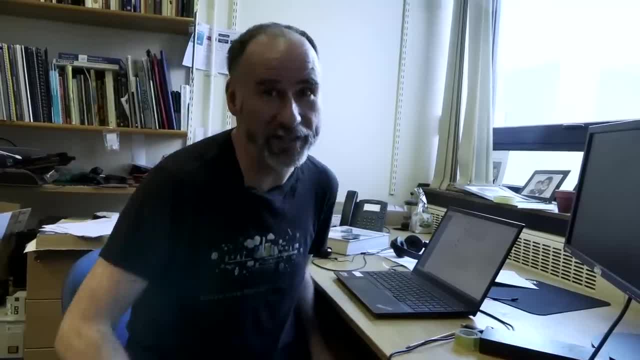 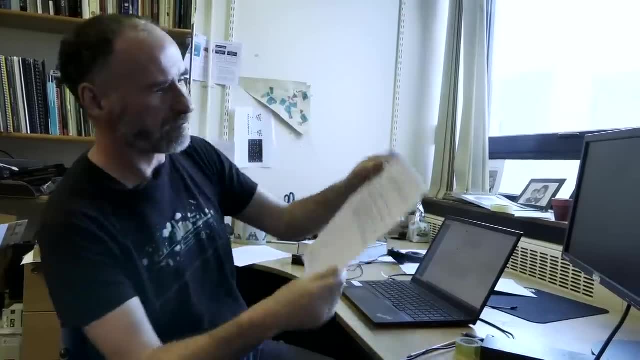 and that's what you're probing in an exam. The whole reason I started looking at this was because a student brought a coursework question to me, typed it in and said: so let me. what I wanna do is ask it. This is a tricky question. 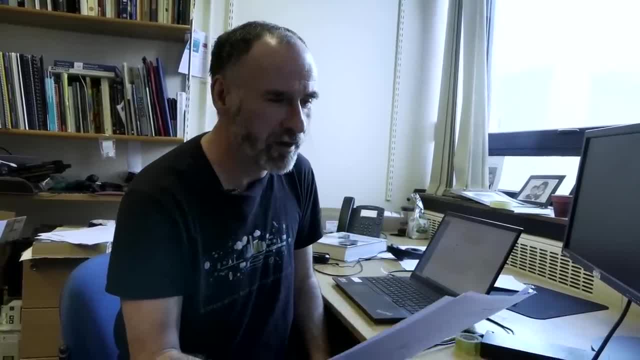 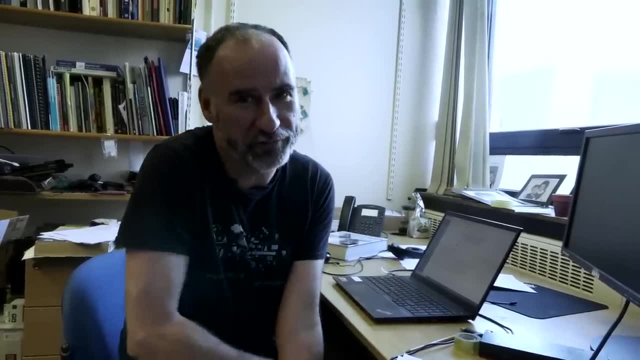 This is a conceptually tricky question by quantum mechanics And I know some of you out there won't have really done a huge amount of quantum mechanics. Some of you will. I know there are a lot of undergraduate students. This is an important question. 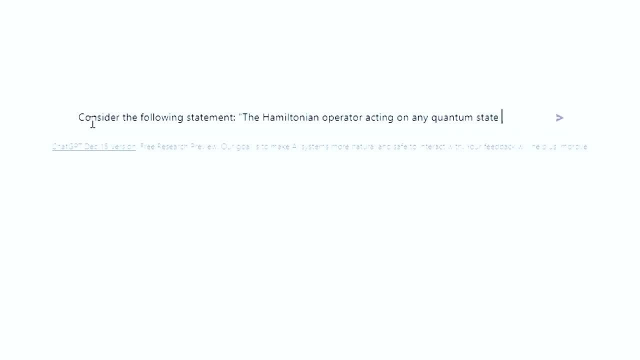 Consider the following statement: Okay, I can't put. I'm not gonna put psi in, I'm gonna call it psi. I'm gonna call the quantum state Y. Consider the following statement: The Hamiltonian operator acting on any quantum state Y. 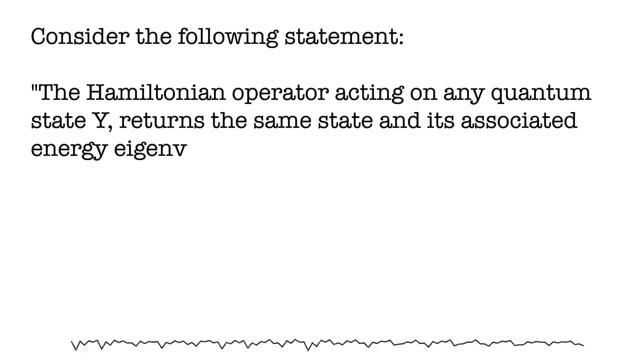 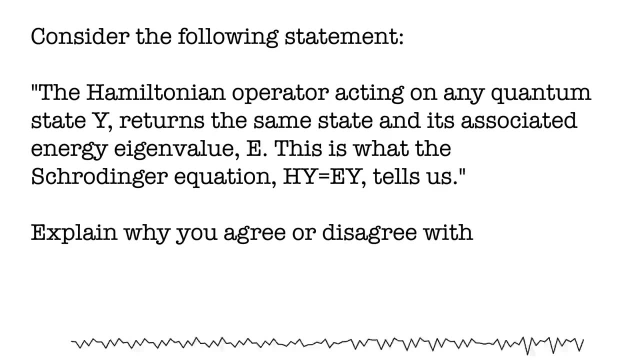 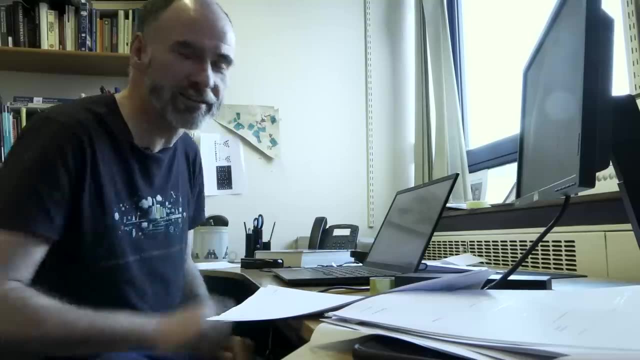 returns the same state and its associated energy eigenvalue E. this is what the Schrodinger equation HY equals EY tells us. Explain why you agree or disagree with this statement. Now I tell the students in the quantum world class that 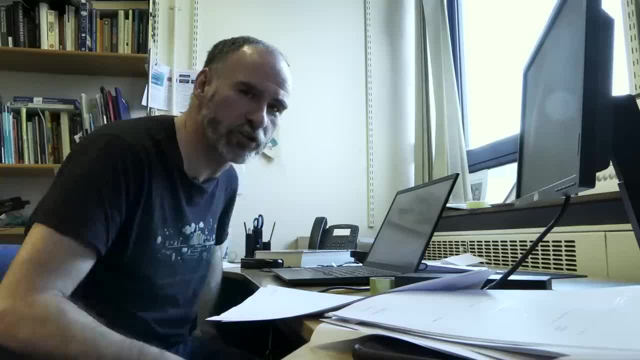 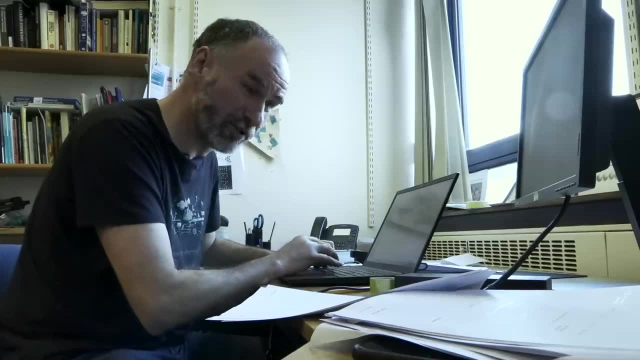 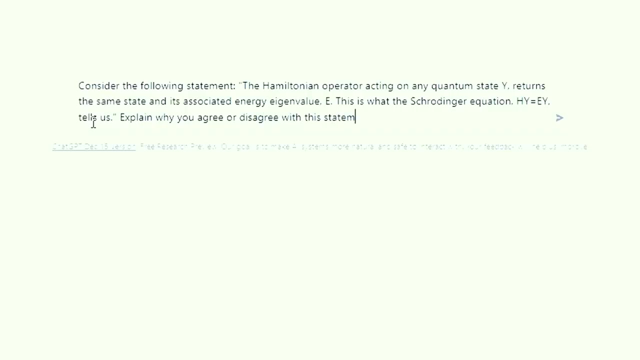 if they come out of the module not understanding and not being able to get the right answer to this question. I've failed. So let's see how ChatGPT does Explain why you agree or disagree with this statement, And there are five marks for this in our marking standards. 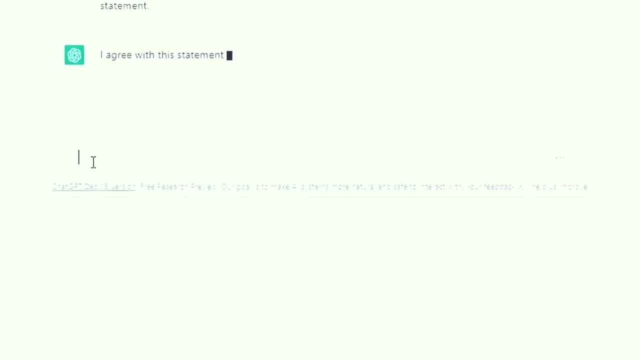 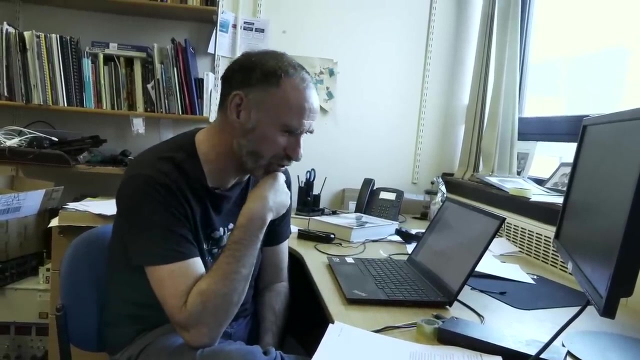 So let's see what ChatGPT does. Ah, wrong. Okay, we could go into details about just why it's wrong, But the important thing is that that's why it's wrong, But the important thing is that that particular equation. 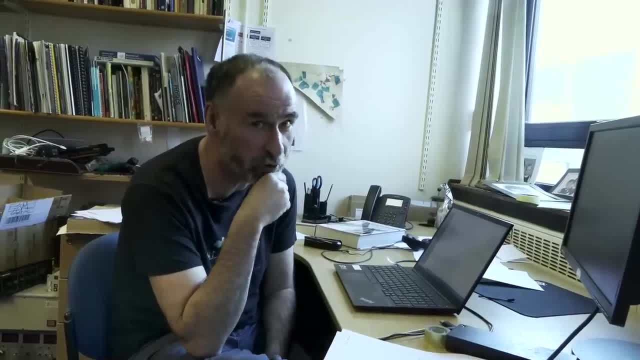 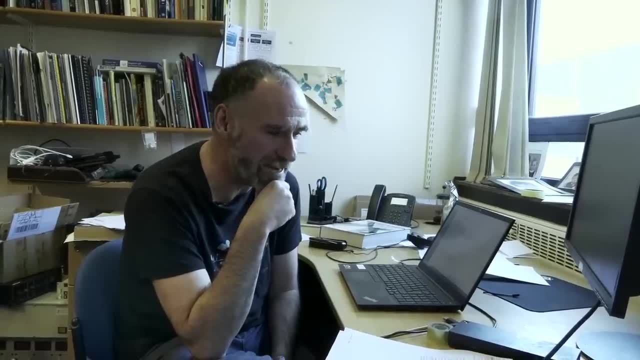 is called the time independence Schrodinger equation. It only works for certain states, what we call stationary states. The question very specifically says: Hamiltonian operator acting on any quantum state. This is exactly what I would hope that students do not tell me. 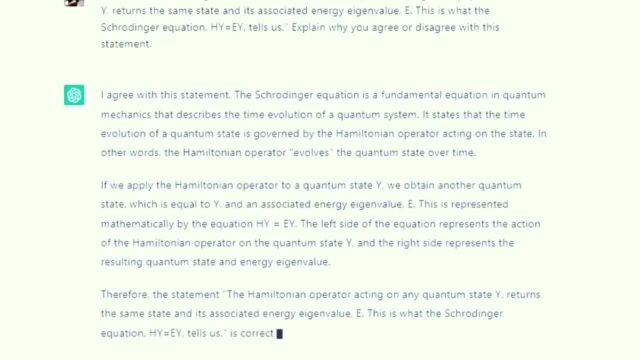 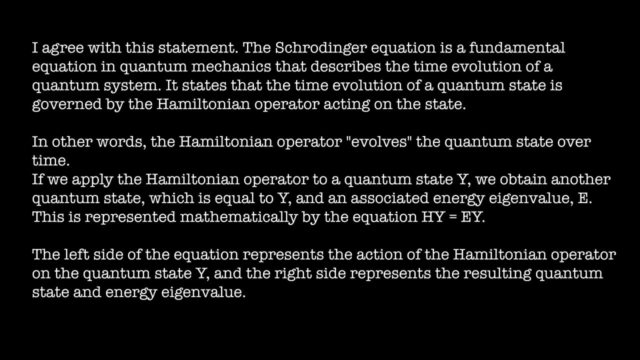 So zero marks ChatGPT- really bad feeling. This definitely needs to go right back to the start of its quantum mechanics knowledge and get a drill. I can point it to some very good online resources about quantum mechanics if it really works. 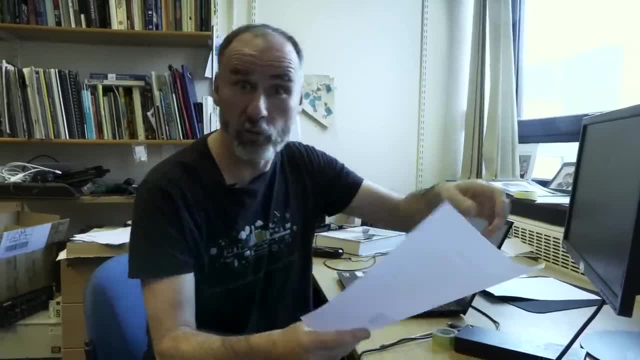 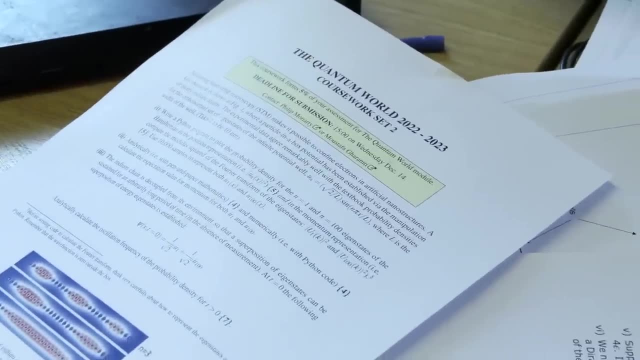 I can point it to some very good online resources about quantum mechanics. if it really works, Okay, quantum world coursework, I'm gonna have to set a new one next year, aren't I? So it's actually about the last computer file video we did. 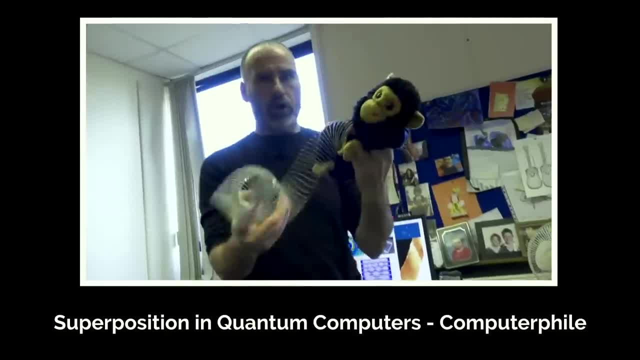 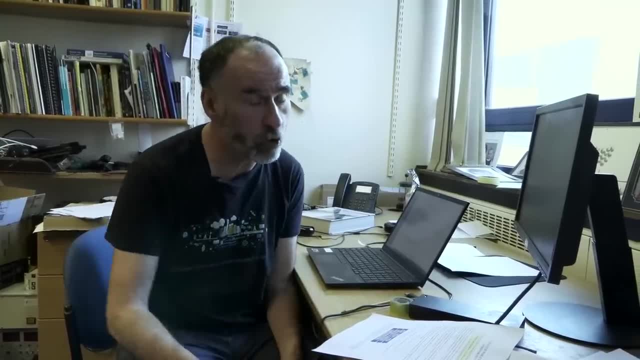 about the superposition. It's a lot of fun to do that one, but it's about particle in a box, superposition of states and what the coursework's asked the students to do. We're trying to integrate more and more computing coursework. 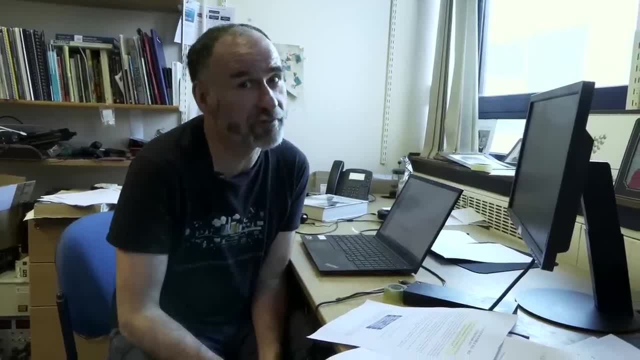 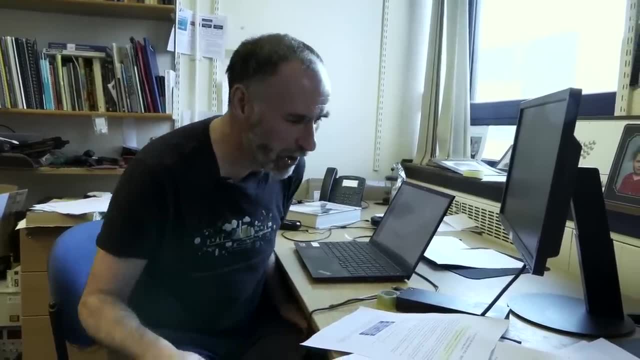 into our physics degrees And because for me computing is equally important, if not more important than mathematics. that's a controversial statement, But write a Python program to plot the probability density for the n equal of one and n equal of 100 eigenstates. 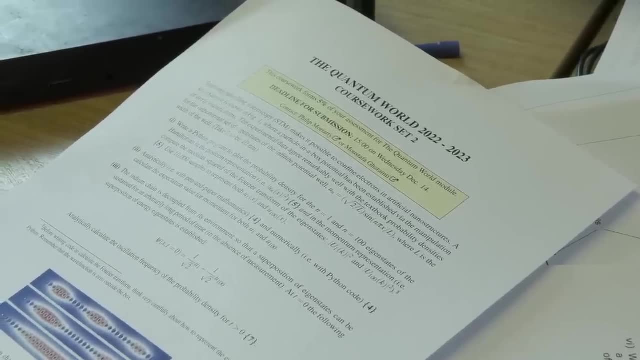 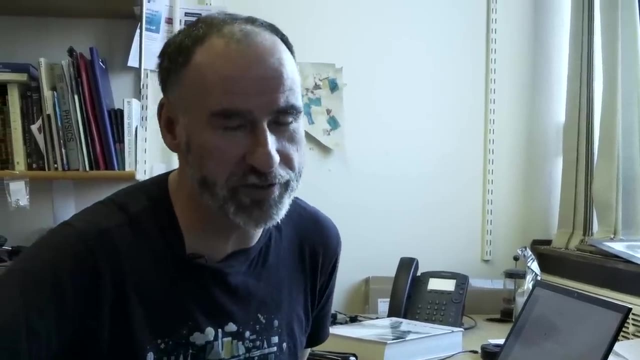 of the Hamiltonian for the infinite potential. well, in the position representation and in the momentum representation, If you're not at second year- possibly end of first year- undergraduate physics level, that's not gonna make a lot of sense to you. But let's just see what ChatGPT does for this. 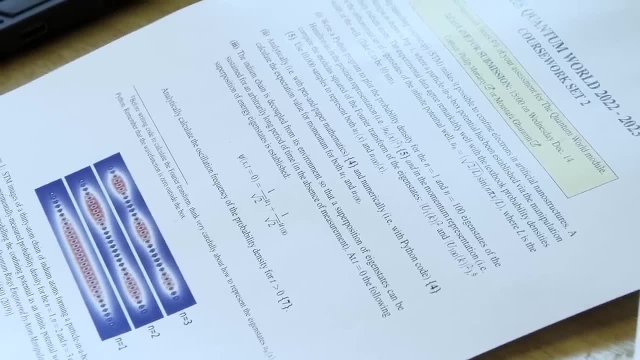 I need to tell it what it is. I need to tell it what it is, So we'll add a little bit. This is not quite the question, I'm just gonna give it a little bit more clout. of the Hamiltonian for the. 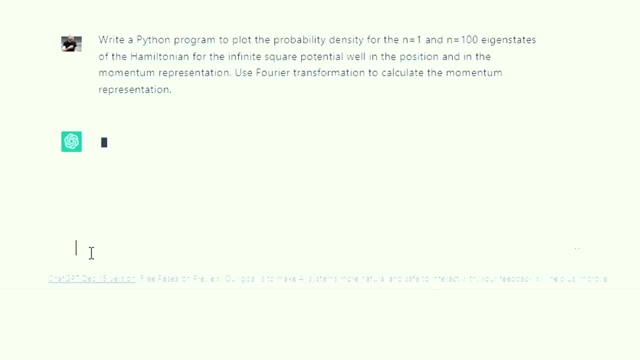 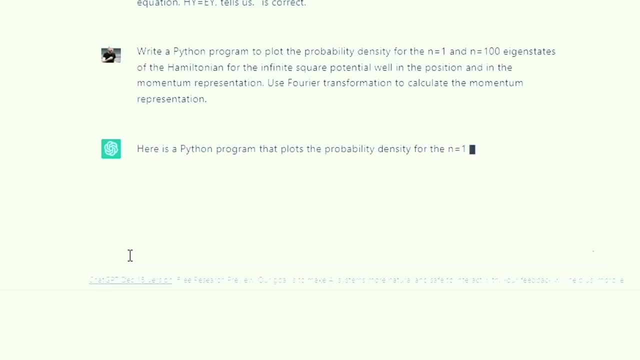 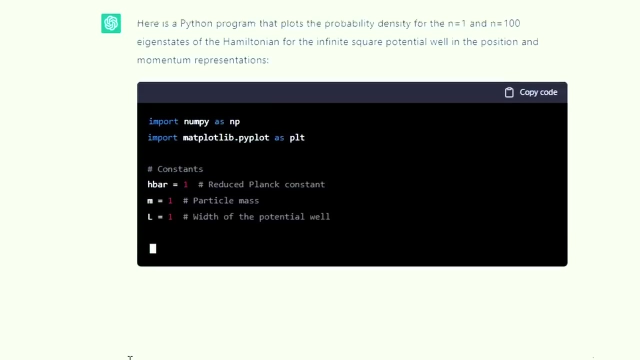 Okay, that's effectively trimmed down version of that question. Let's see how it does. This requires a lot of conceptual understanding. Oh, here's a okay. Okay, good start. Okay, it's using appropriate units. Okay, that's fine. 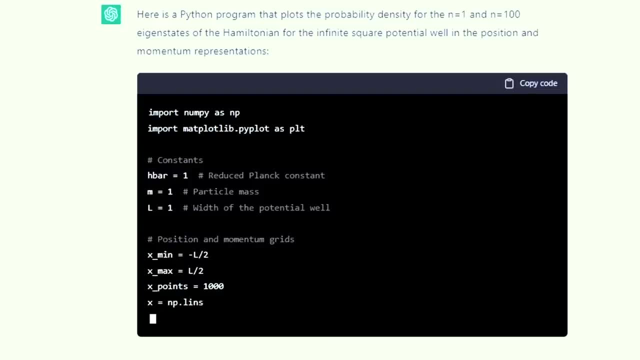 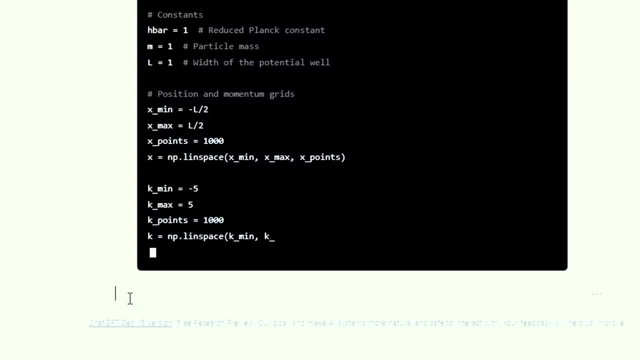 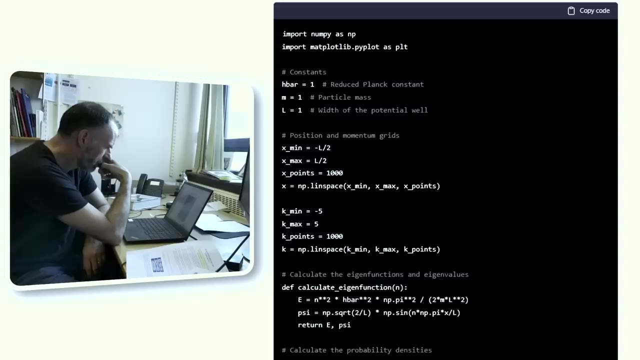 Good, Oh, it's done it that way. Okay, Thousand points might be quite enough for something which is oscillating as high as that higher eigenstate, But okay, let me scroll down. That's interesting. It's putting the energy eigenvalue. 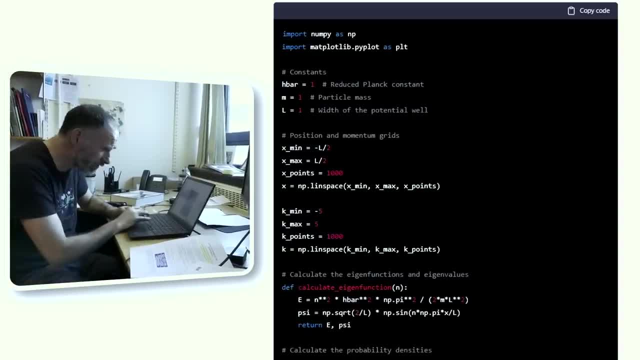 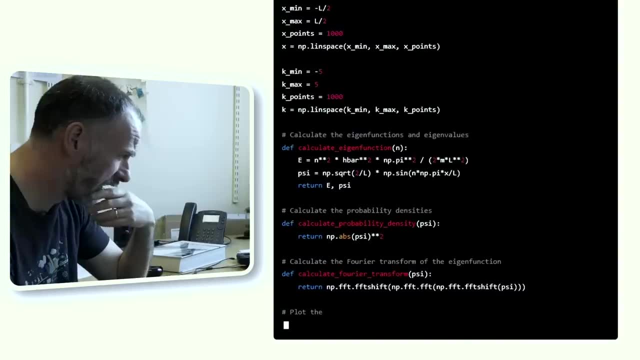 in as well as the eigenfunction Probability density. Then it's gonna calculate the Fourier term. Oh my God, this is bloody hell Good. No, it's. yeah, It's scarily good In terms of doing the coding. 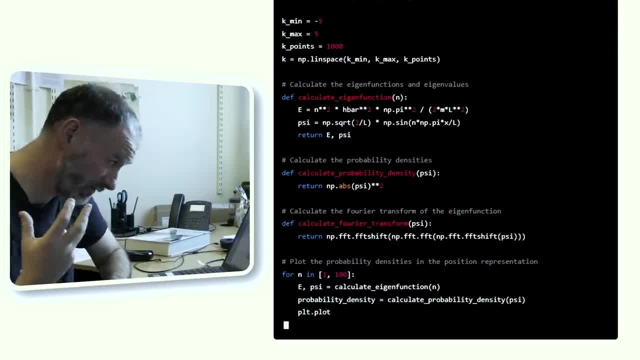 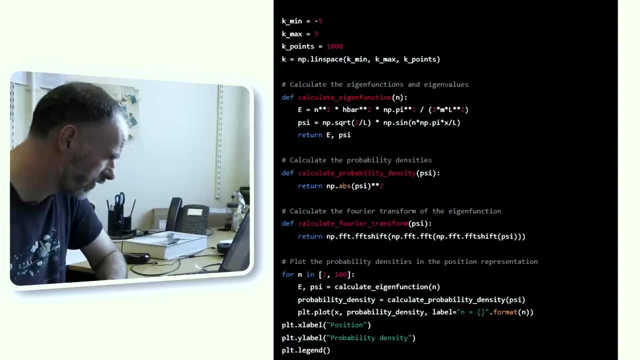 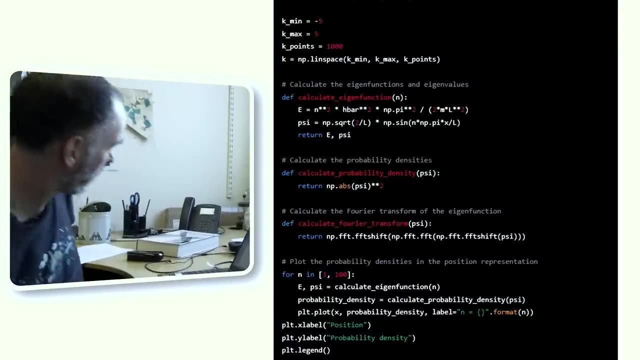 it hasn't quite got, it's exactly. it's made the exact mistake I'd hope the students wouldn't make, But in terms of the overall structure of the code that is pretty impressive, And it's even FFT shifted it, Wow, okay. 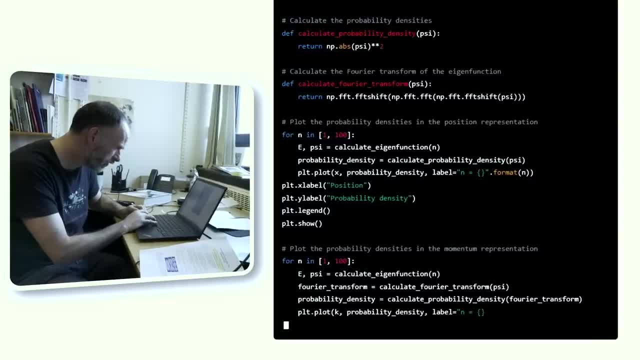 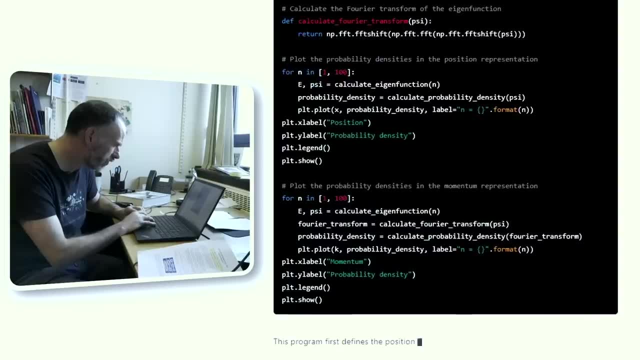 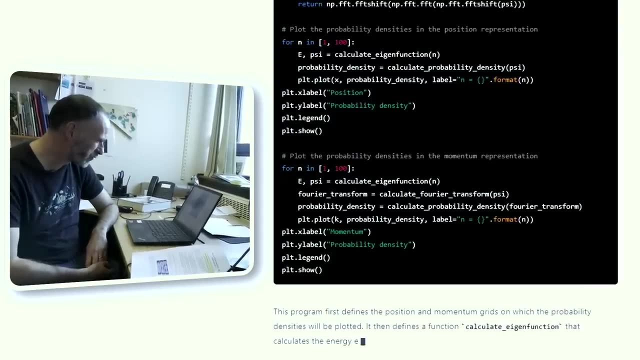 And then what's it doing? It's trying to. is it still going? It is, So it's now explaining what it's done. The program first defines the position of momentum grids on which the probability densities will be plotted. Okay, so we'll leave it going. 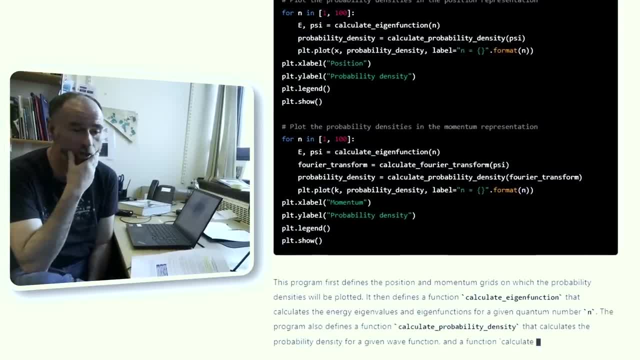 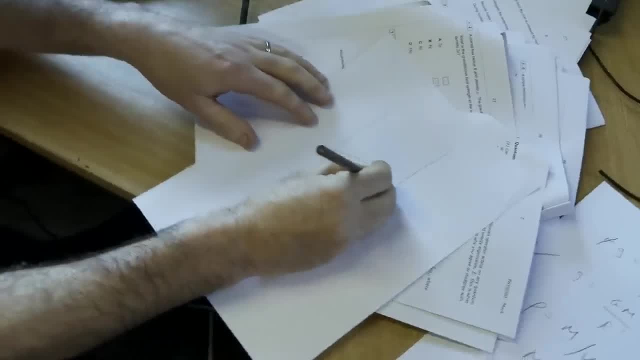 churning away in the background. That's pretty impressive. The one issue, however, is that the reason I set that question is it requires careful thought. So what we have? this thing as ever, which, even if you haven't done, quantum mechanics. 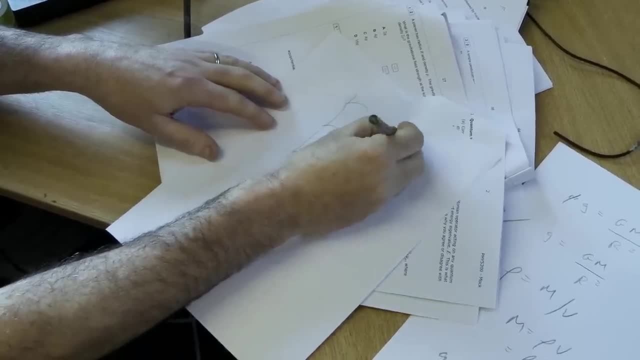 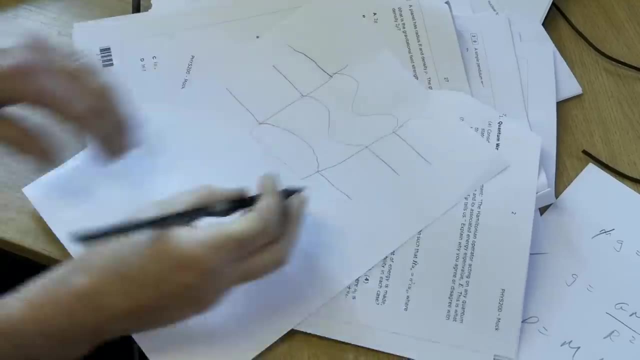 you'll recognize this in terms of standing waves on a string. That's what we're talking about. Important aspect of this is that in each case, those functions go to zero outside the well. What it's done is it's just assumed that those sine functions continue on outside the well. 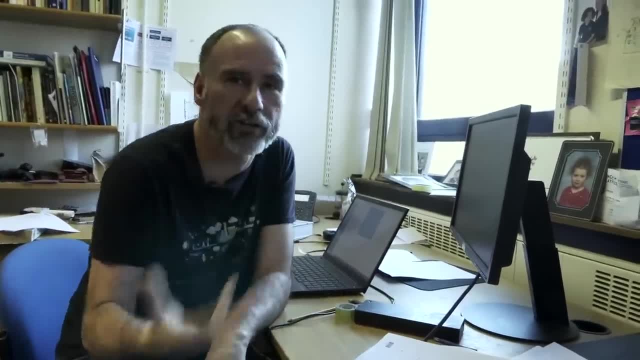 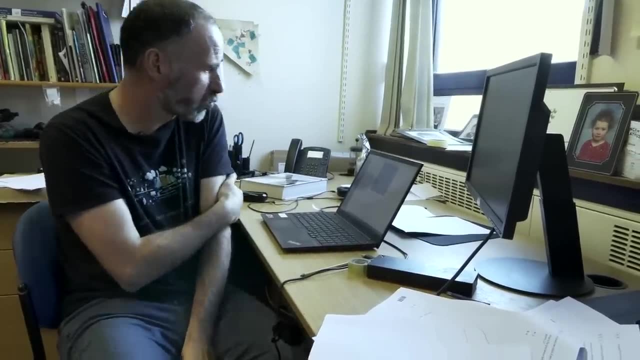 That's exactly this mistake I don't want students to make, because that doesn't give you the right momentum representation. So it's performed as well. as a student that has a good understanding of coding and very good understanding of coding, Very good understanding of coding, I would say. 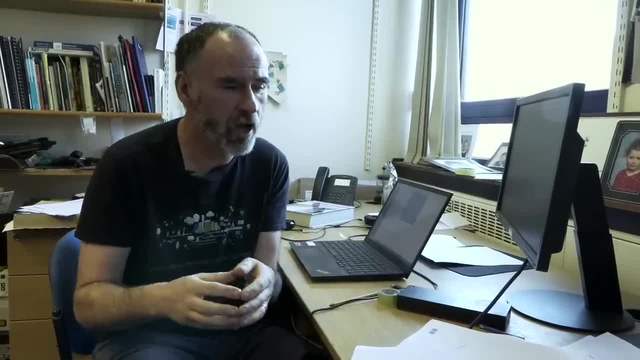 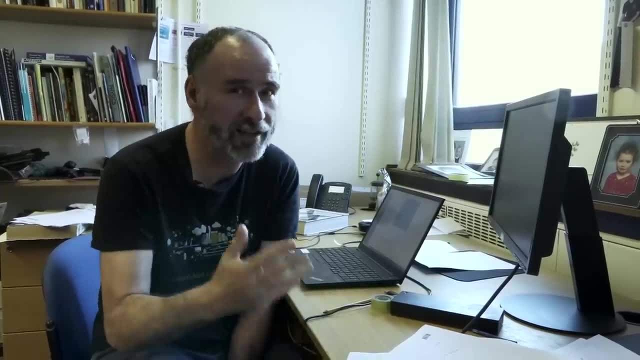 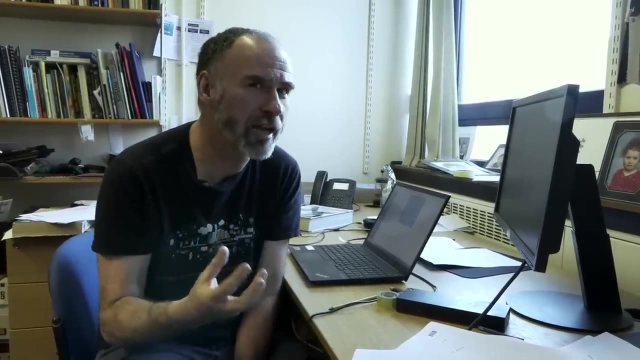 but not such a great understanding really of the physics of this problem. They understand a lot of the physics but not quite enough and they've made exactly the mistake. I say they anthropomorphizing there. ChatGPT has made the same mistake. I would expect. 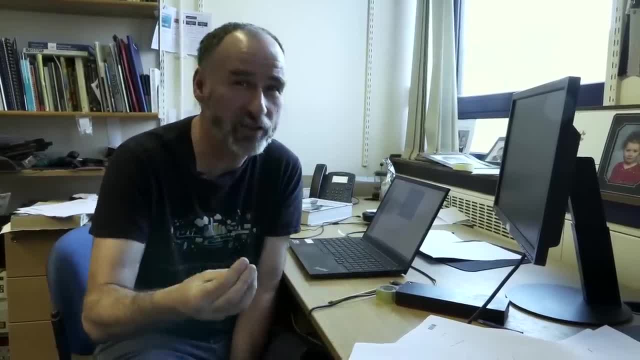 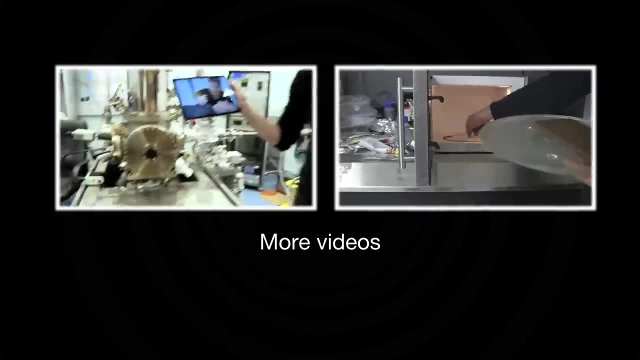 and would hope that many students wouldn't make- So it's failed- the sort of conceptual test here again. If we could influence matter at the subatomic level by clicking our fingers, we wouldn't have to spend billions on CERN, We wouldn't have to. 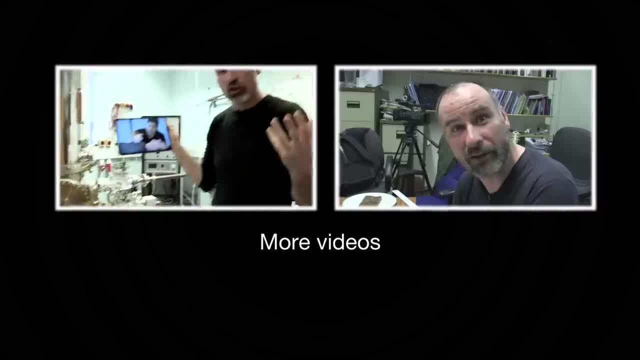 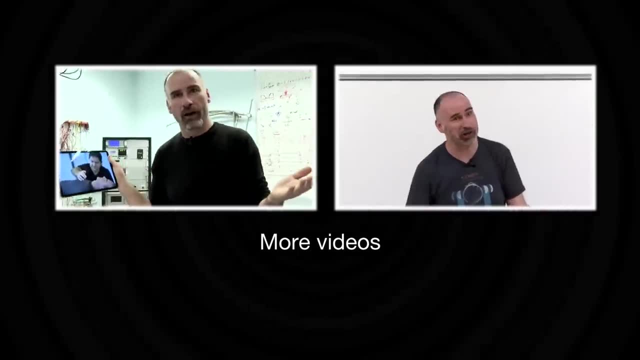 And we wouldn't need this bloody thing. No, this is just nonsense. This really is just nonsense, And the argument will be made: well, science doesn't know everything, so how do you know? Sure, science doesn't know everything.